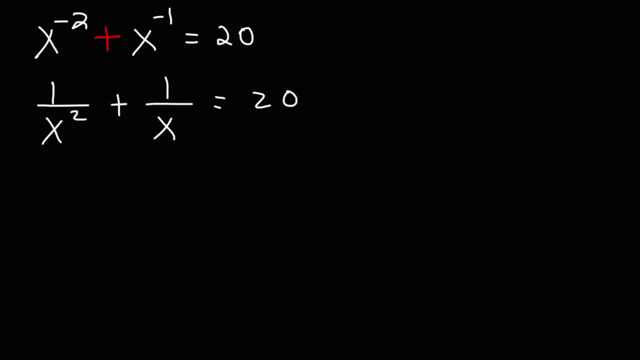 The next thing that I recommend doing is getting rid of the fractions. We want to multiply every term by x squared. So we're going to multiply the first fraction by x squared and the second fraction by x squared, And whatever you do to the left side of an equation, you must also do the same to the right side of the equation so that the value doesn't change. 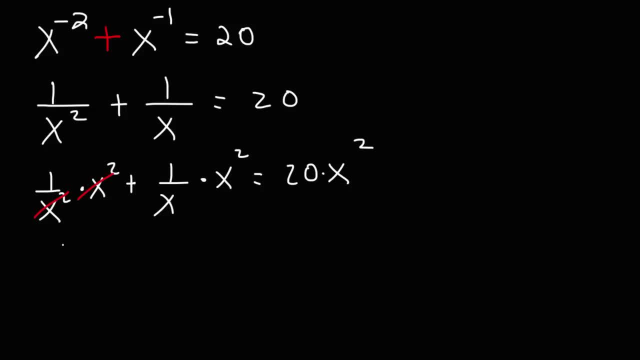 1 over x squared times x squared is simply 1.. 1 over x times x squared, that's basically x squared divided by x. that's equal to x. You can think of x squared as x squared divided by x, Or you can think of x squared as being the multiplication of two x's or two x variables together. 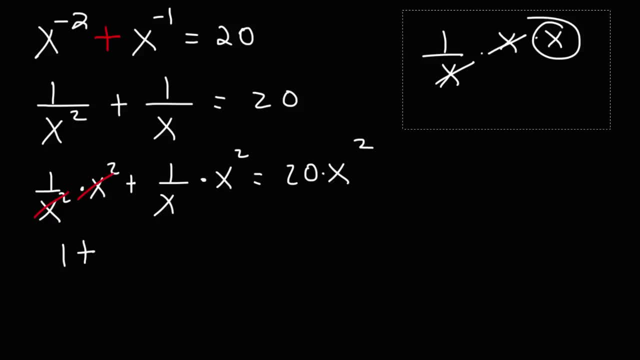 So 1 cancels and we have 1 left over. So we just have plus x and that's equal to 20x squared. Now what we need to do at this point is subtract both sides by x and negative 1.. 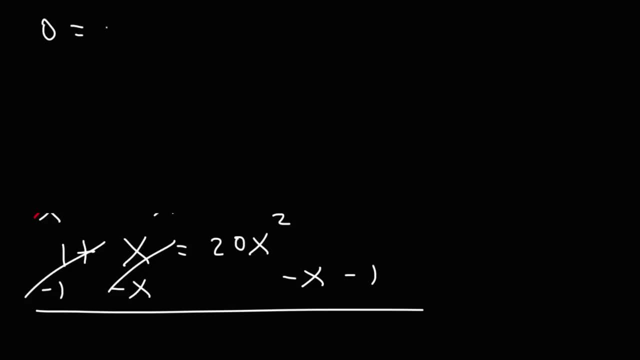 So what we're going to have at this point is 0.. 0 is equal to 20x squared minus x minus 1.. So now that we've reached this point, what is our next step? What we have here is a trinomial where the leading coefficient is not 1.. 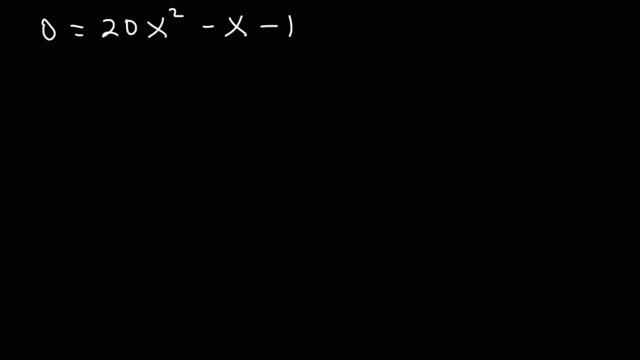 In order to solve this quadratic equation, we can either factor the trinomial or use the quadratic formula For this problem. I'm going to factor it. So what we're going to do is we're going to multiply the leading coefficient by the constant term. 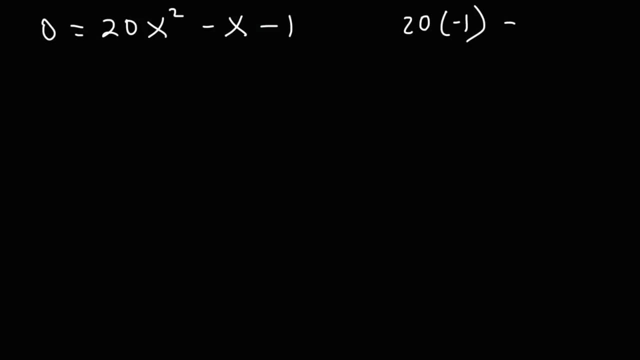 20 times negative 1 is negative 20.. And we need to find two numbers that multiply to negative 20, but add to the middle coefficient negative 1.. So what two numbers multiply to negative 20, but add to negative 1?? 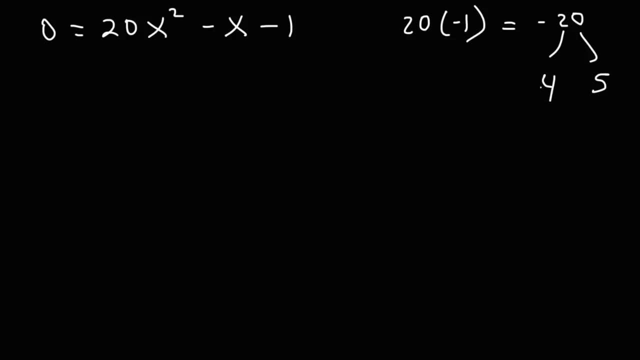 Well, this is going to be 4 and 5.. But positive 4, negative 5.. 4 plus negative 5 adds up to negative 1, but these two numbers multiply to negative 20.. So we're going to replace negative x with negative 5x plus 4x. 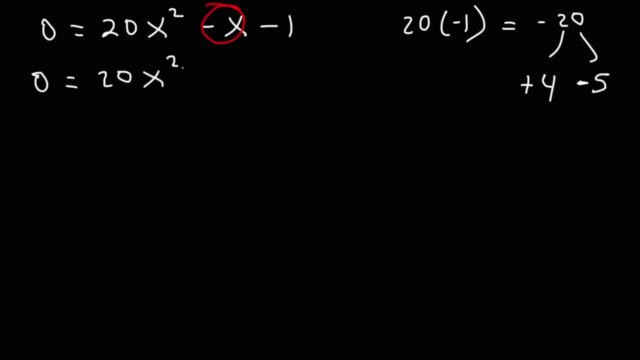 So we have: 0 is equal to 20x squared minus 5x plus 4x minus 1.. Now we need to use a technique called factoring by grouping. In the first two terms, we're going to take out the GCF. 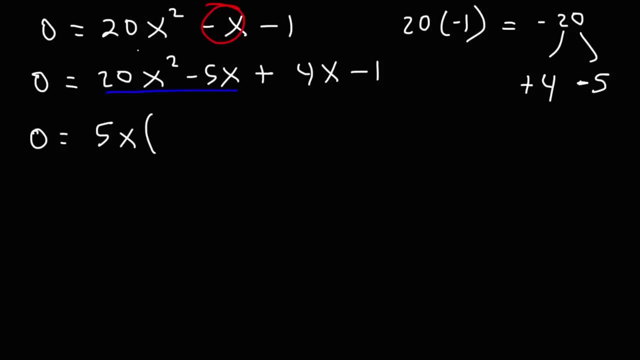 The greatest common factor, which is 5x. 20x squared divided by 5x, that's 4x, And if we divide these two, that's going to be negative 1.. Now there's no GCF that we can take out for the last two terms, so we're just going to factor out 1.. 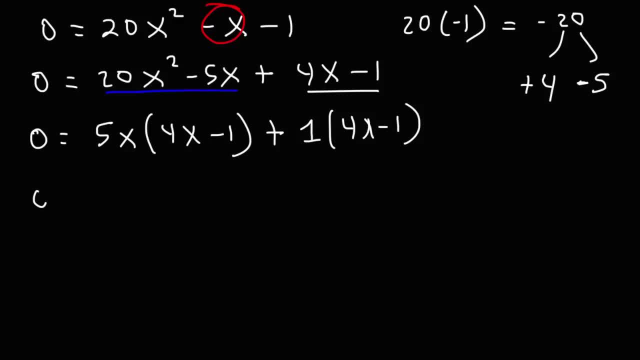 So we have 1 times 4x minus 1.. Our next step is to factor another GCF. In this case that's going to be 4x minus 1.. Outside of that, we have 5x plus 1.. 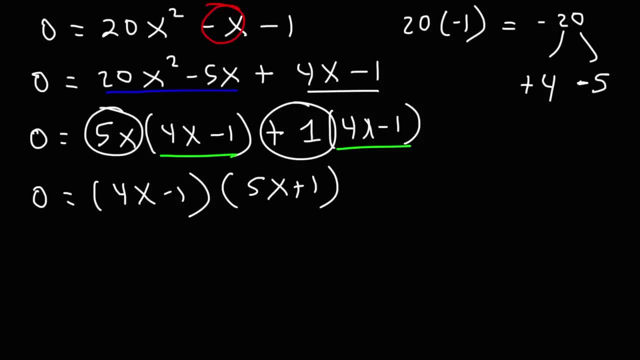 So that goes here. So that's how we can factor 20x squared minus x minus 1.. Now, using the zero product property, we're going to set each of these two factors equal to 0.. So that's 4x minus 1 is equal to 0.. 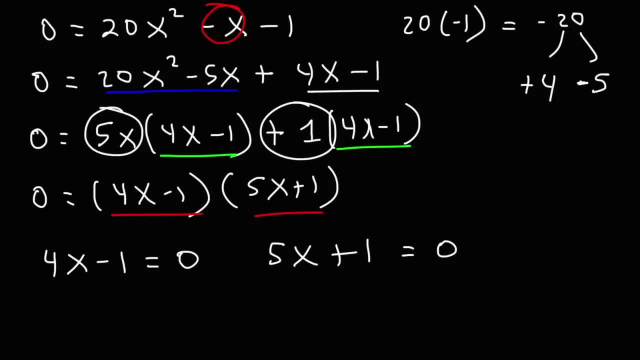 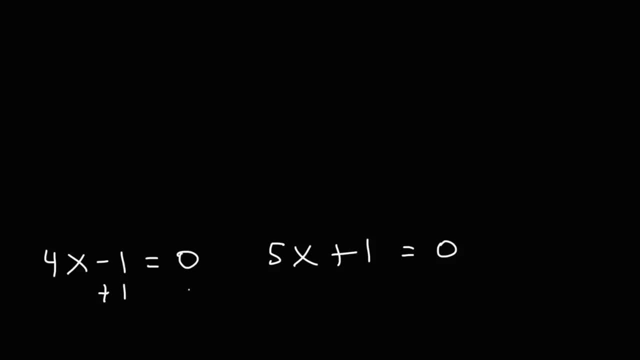 And 5x plus 1 is equal to 0.. Now let's solve. So. in the first equation I'm going to add 1 to both sides, So I get 4x is equal to 1.. Next I'm going to divide both sides by 4.. 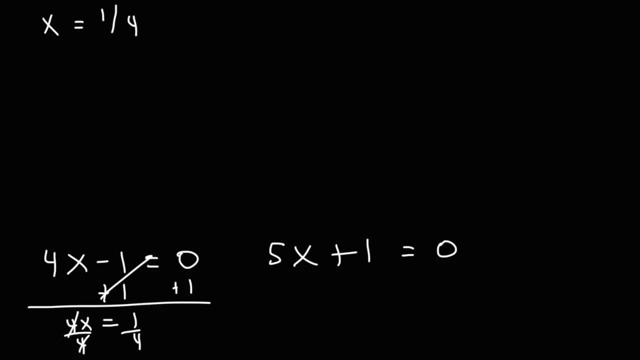 So this gives me the first answer: x is equal to 1 over 4.. For the next equation, I'm going to subtract both sides by 1. So I get 5x is equal to negative 1. And then divide them. 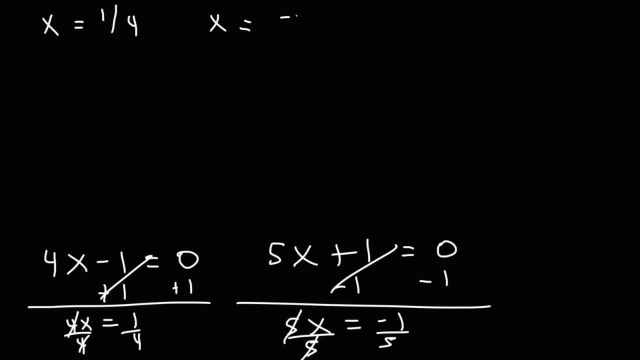 So I get: 5x is equal to negative 1 over 5.. I have another potential answer: x is equal to negative 1 over 5.. So now what we're going to do is we're going to check these two answers. 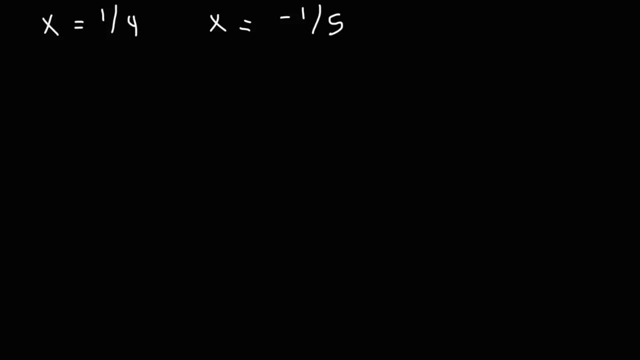 Because both of these values may be correct answers, Or one of them might be correct, Or none of them might be correct. So let's find out, just to make sure. So here is the original equation. So let's start with 1 over 4.. 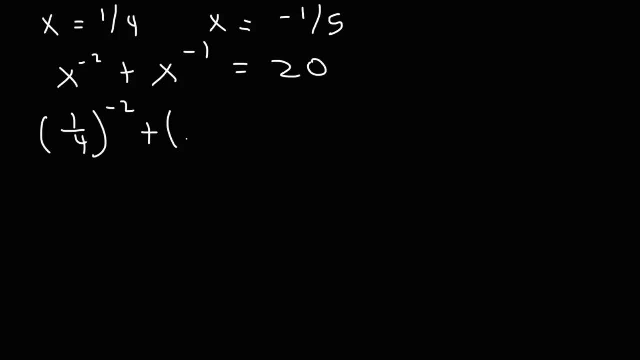 Let's replace x. Let's replace x with that number. Now, what is 1 over 4 raised to the negative 2nd power? Well, first let's apply the negative exponent To change the negative 2 into a positive 2, we need to move the 4 to the top. 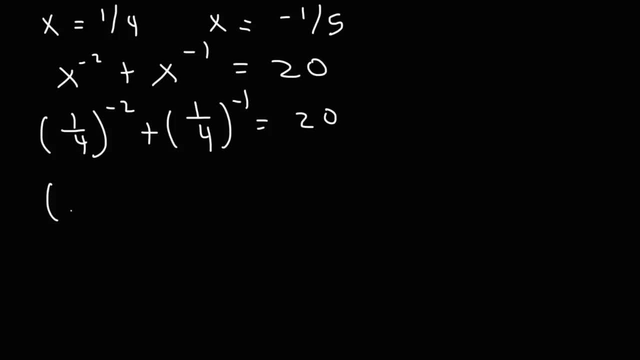 So basically, 1 over 4 becomes 4.. 1 over 4, raised to the negative 1., Is just 4.. But for those of you who want to show your work step by step, here's what you can do. 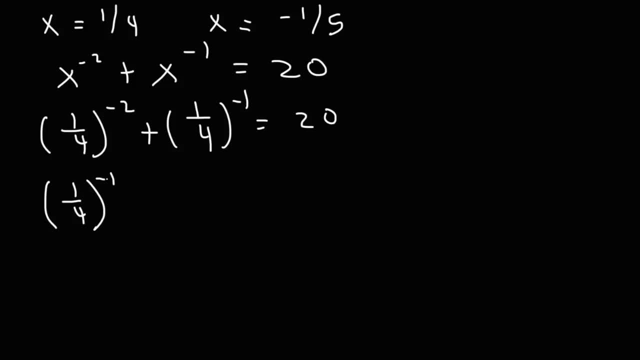 You can write negative 2 as being negative 1 times 2.. When you raise one exponent to another, you need to multiply. So now 1 fourth raised to the negative 1, power is just 4.. So we have 4 squared. 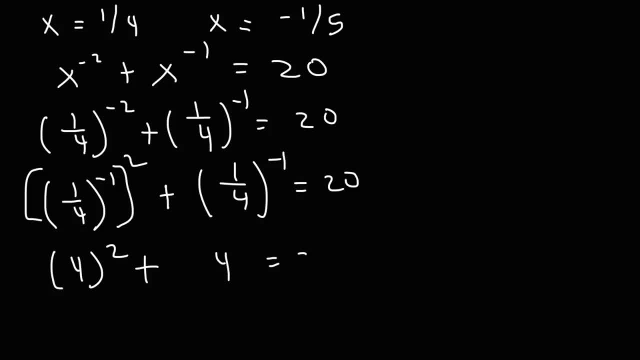 And this is the same. That's going to be 4 again, And then 4 squared, or 4 times 4, that's 16.. So we have 16 plus 4, which is 20.. And so we can see that this is certainly one of the answers. 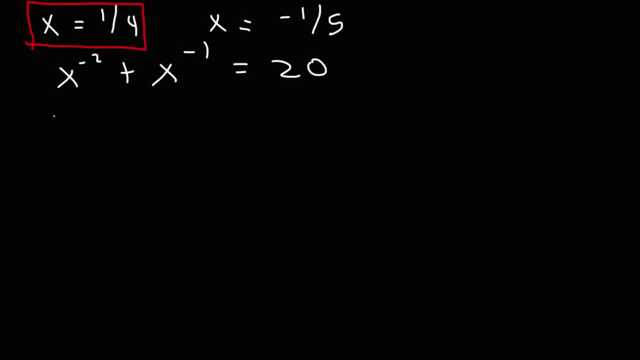 Now let's check the other answer. So let's replace x with negative 1. Over 5.. So we're going to follow the same process. We're going to break down negative 2 into negative 1. Raised or times 2.. 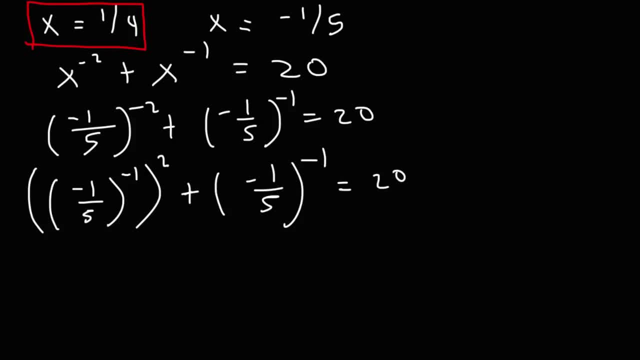 Negative 1 over 5 raised to the minus 1.. We just got to move the 5 from the bottom to the top, just like we did with the 4. So negative 1 over 5 raised to the negative 1st power. 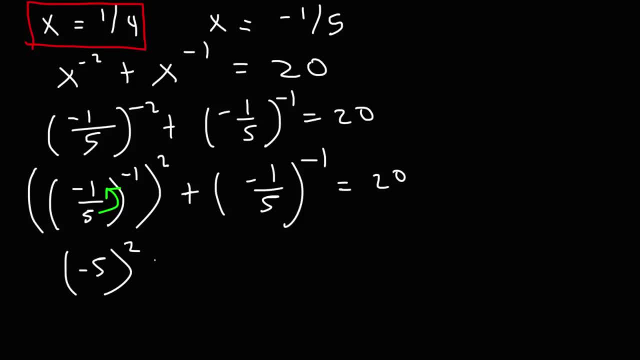 That's going to be negative 5.. So we have negative 5 squared plus another negative 5. And that's equal to 20.. Negative 5 squared, That's negative 5 times negative 5, which is positive 25..